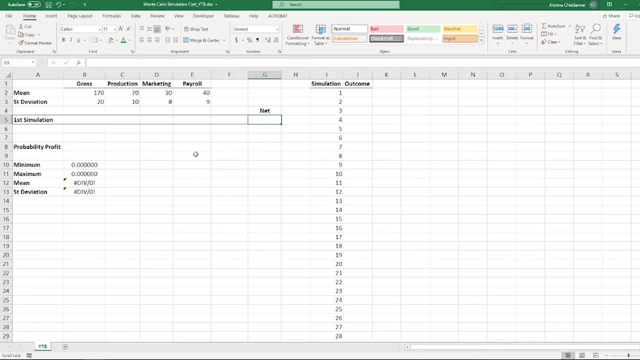 produce a net income. We'll repeat the simulation 500 times and we'll use an excel tool called the data table to do it. Imagine you have a manufacturing business or a construction project in progress and your average gross monthly income is in thousands of dollars in cell B2.. 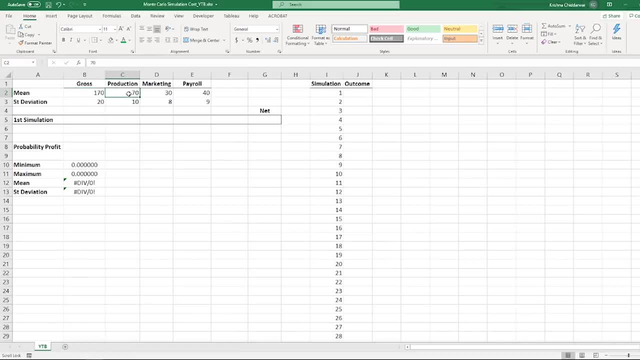 Your average production cost is in C2.. Average marketing cost is in D2 and your payroll is in E2.. The corresponding standard deviation for each of these figures is in row 3.. Standard deviation is a statistic that measures how far your values can deviate from the mean. Let's assume that these 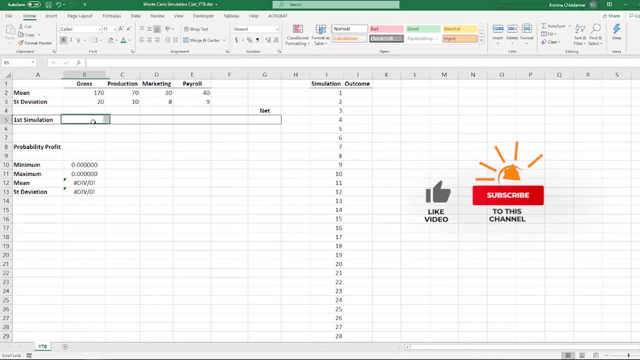 numbers are normally distributed for now. Now, before we move on to our first simulation, I would really appreciate if you like this video and share it with your friends and family. Like this video and subscribe to my channel. Let me know in the comment section if this video has. 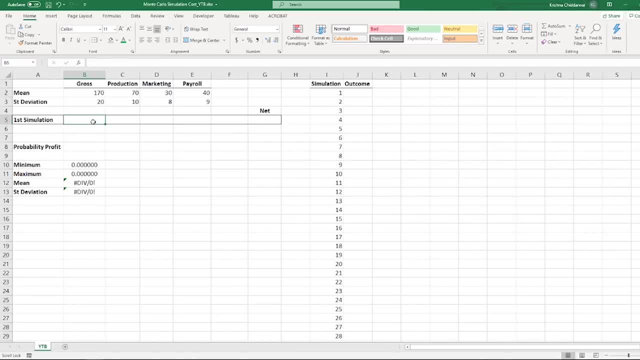 been of any use to you. So let's move to our first simulation in row 5.. First thing to do is to generate a random number for gross meaning, a number randomly selected from a normal distribution whose mean is 170 and whose standard deviation is 20.. In cell B5, type equal: norminv- left bracket. 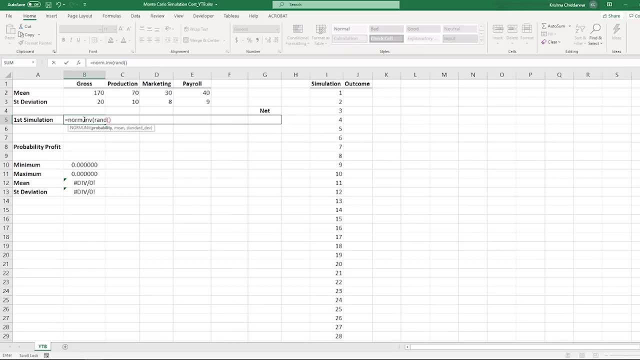 rand open, close comma and cell B2 comma. cell B3, right bracket. The rand function gives us a random number between 0 and 1 and the function uses that as a probability, with B2 and B3 as mean and standard deviation. Let's drag the formula over to the right to column E for the remaining results. Next we need to think: 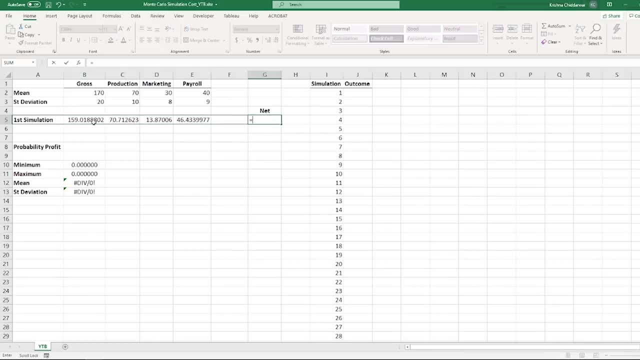 about the net income, Everyone's bottom line right? Well, that's just the gross income minus the sum of the cost. So in general the net income is the sum of the cost. So in general in B5, if we run a simulation, B5 is like this: in G5, that's equal b5 minus sum of c5 through and e5,. 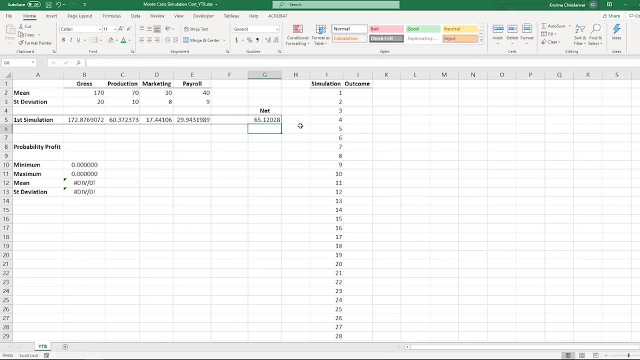 and that's the result of 4 simulation. I've defined outcomes for the rest of 500 trials as the range of cell J1 through J5 O1. now, before we run a simulation 500 times and calculate the net income each time- note the statistics will be calculated after the simulations are done- cell B8 will show: 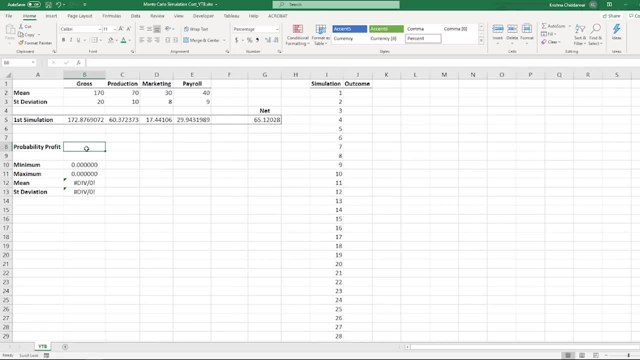 the probability of making a profit. That's the proportion of times the net income is positive. So So in B8, type: equal countif left bracket outcome comma quote greater than zero. unquote right bracket divided by 500.. 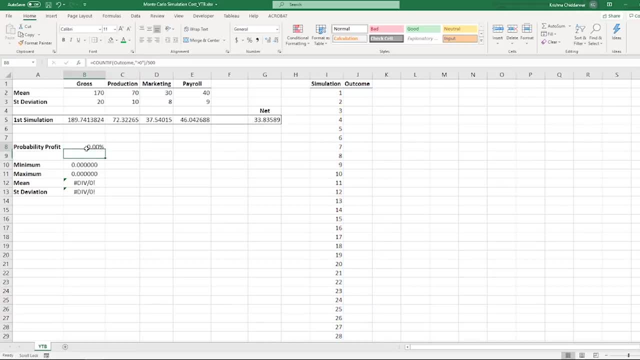 Which is the total number of trials for which we are running a simulation. The other statistics are pretty straightforward. Minimum in cell B10 will show the least amount of net income generated. Maximum in cell B11 will show the maximum profit that could be generated. 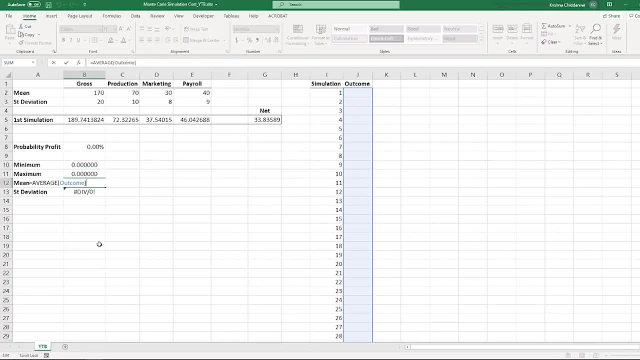 Mean in B12 will show the average profit generated by a business or project And, in the end, a standard deviation in B13, which will show how far your values can go from the average profit number. For now, you'll see some error messages in B12 and B13 before we start our simulations. 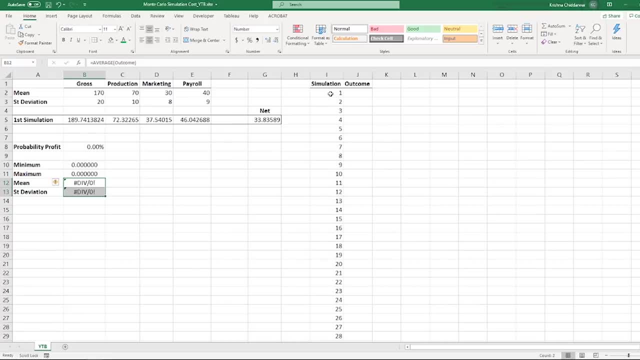 The data table and the 500 simulations will appear. in outcome We get the first one from G5.. So in J2, type equal and select G5.. Now I have to highlight the area. That will be the data table. So select I2 and J2 and fill up the area. 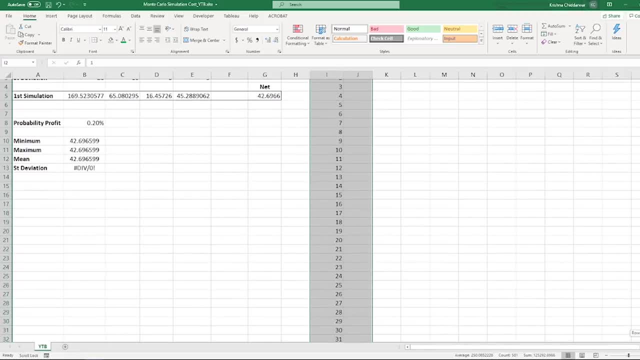 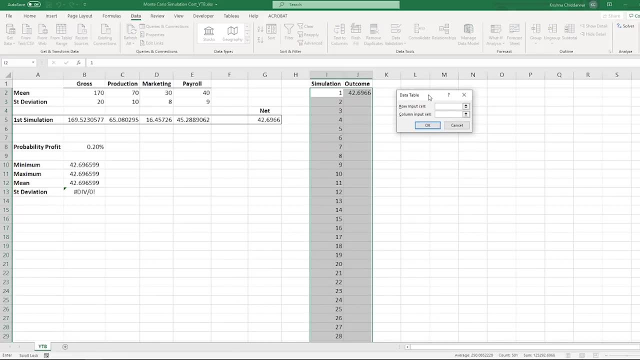 Scroll back up On the data tab. in the forecast area, select what if? and data table In a dialog box. row input cell doesn't mean anything to us in this context, So leave it blank. Column input cell does matter, So click in input cell and all we have to do is to select a cell which is not in the range of the data table. 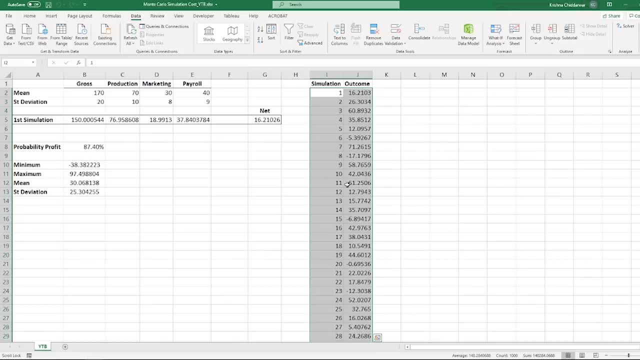 Click OK And the data table fills up with the outcomes of 500. And the statistics fills in too. You can see the minimum, the maximum mean and the standard deviation, And you can also see the probability of generating a profit on your business. 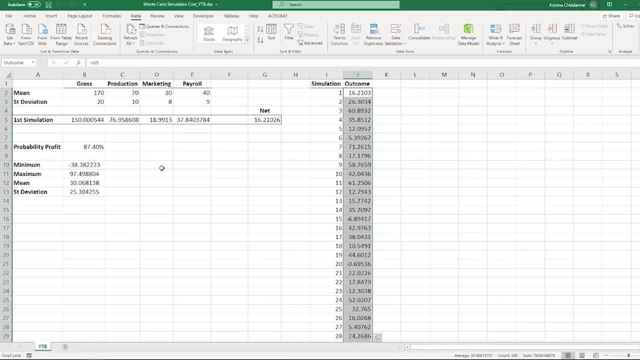 Now remember one thing: Each time you do something significant on the spreadsheet, these 500 simulations will run again. We can also take a look at the distribution of the simulation outcomes. For that, highlight the data in column J and then insert a histogram. 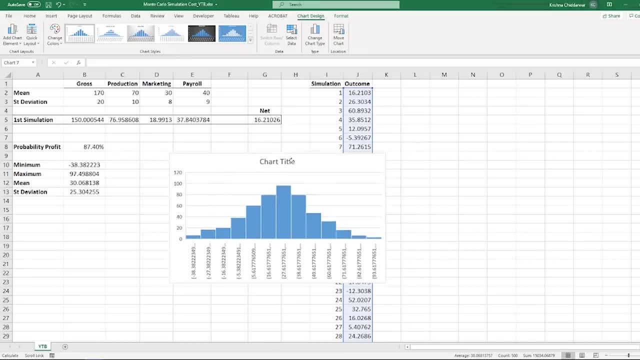 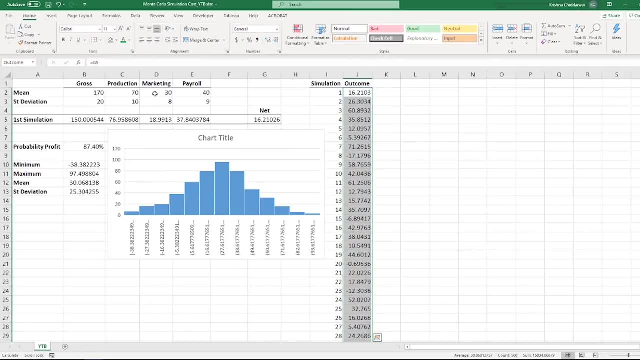 This gives you a look of the distribution of outcomes. Want to see what happens when you change some of the inputs. Suppose you decide to increase the marketing cost, let's say from 30 to 50. Take a look at what that does to the probability of profit.